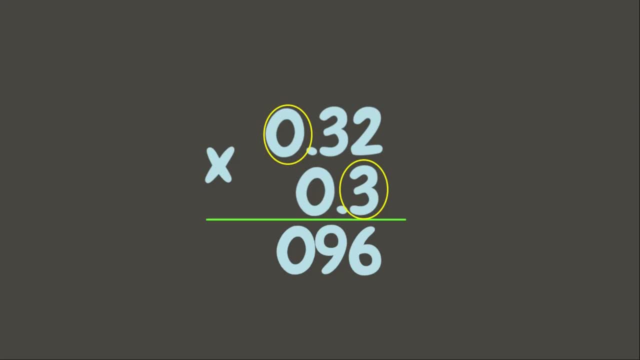 multiply it. Now. is this our final answer? Not yet. We need to put the decimal point in the right place. The next step that we need to remember is: the total number of decimal places in the factors should be the same in the product. Let us count the decimal places in the factors 1,, 2, and 3.. 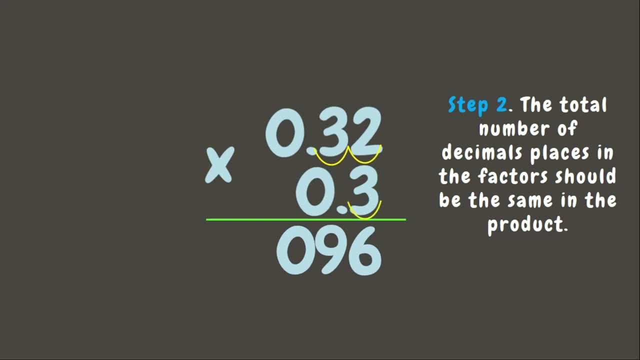 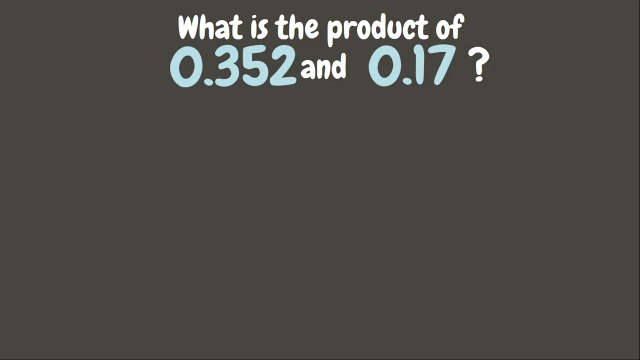 Therefore, we need to put the decimal point in the product three decimal places from right: 1,, 2, 3.. There Let's put 0.. Now, this is our final answer. Let's have another example. What is? 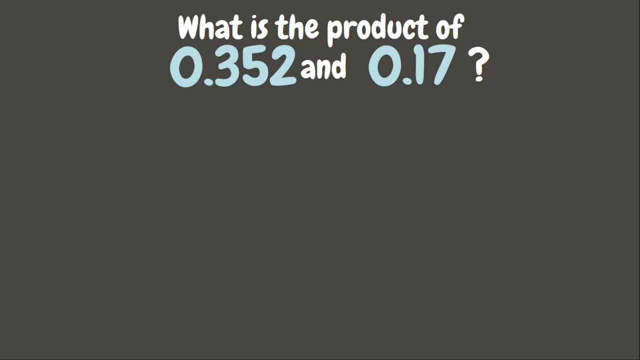 the product of 352 thousandths and 17 hundredths. When we are looking for the product, it means we need to multiply 7 times 2 is 14.. Write 4.. Carry 1 to the next place value. 7 times 5 is 35. Plus 1 is 36.. Write 6.. Carry 3 to the next place value. 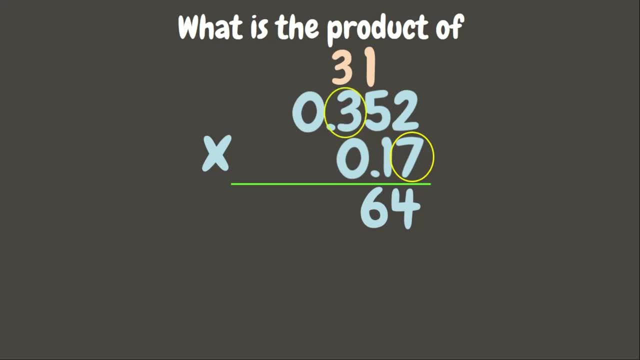 7 times 3 is 21 Plus 3 is 24. Write 4, carry 2 to the next place. value 7 times 0 is 0 Plus 2 is 2. Next one: 1 times 2 is 2. 1 times 5 is 5. 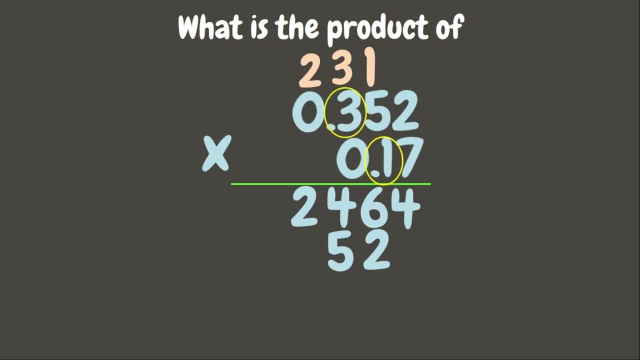 1 times 3 is 3 And 1 times 0 is 0, Since the next digit is 0, we don't have to multiply it Now. let's add the products: 4. Bring down 4. 6 plus 2 is 8. 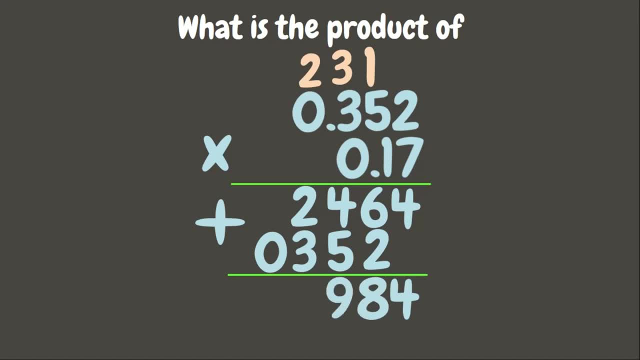 4 plus 5 is 9, 2 plus 3 is 5, And bring down 0. Now remember, the total number of decimal places in the factors should be the same in the product. So let's count 1, 2, 3, 4. 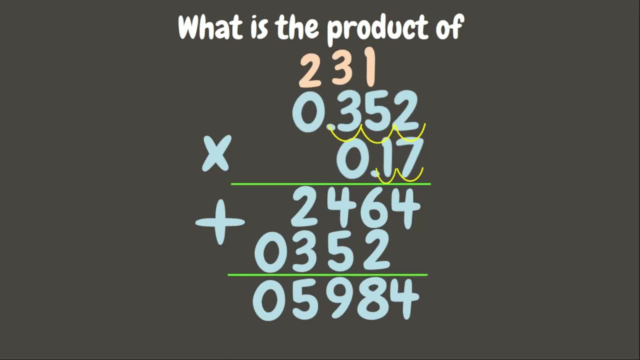 5. Therefore, we are going to put the decimal point in the product. 5 decimal places from the right: 1, 2, 3, 4, 5, There- and let's put 0 Now. this is our final answer. Let's try another one. 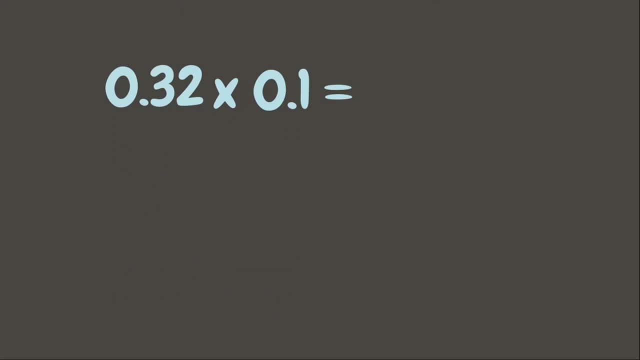 32 times 3 is 2, 2 twice 7, 22 hundredths Times 1.. 1 tenths. And multiplying decimals by 1 tenths or 1 hundredths, The first thing that we need to do is to copy the factor. 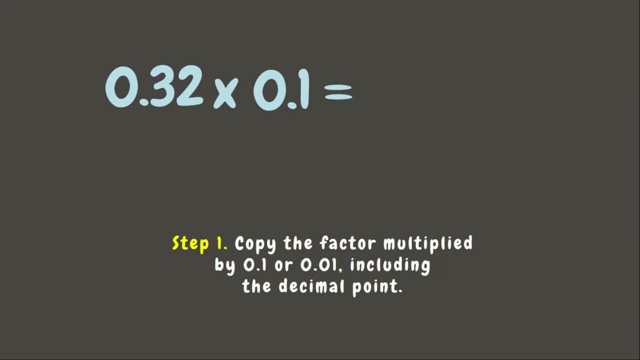 Multiply by 1 tenths or 1 hundredths, Including the decimal point There, And then the next step is The number of decimal places in 1 tenths or 1 hundredth means the number of decimal, the number of decimal places. you move the point to the left, since 1 tenths has. 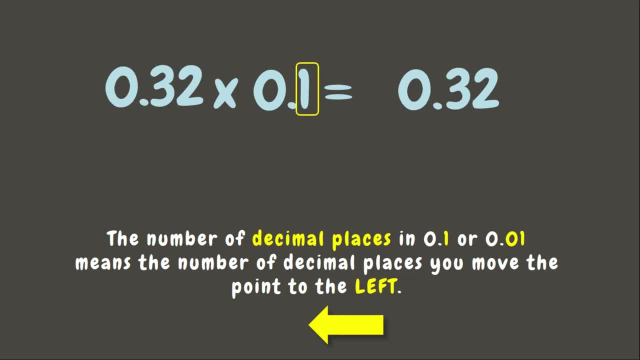 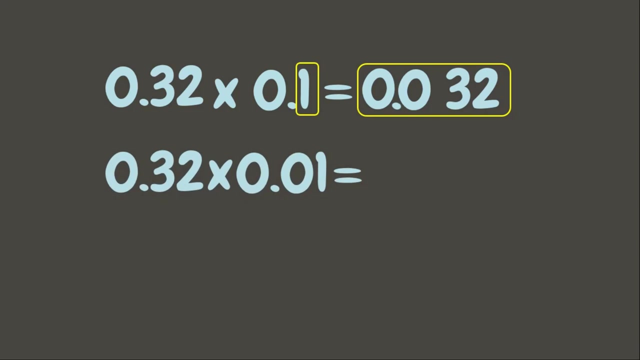 one decimal place. therefore, we are going to move the decimal point one place to the left. there let's add 0. now this is our answer. let's have another one: 32 hundredths times 1 hundredths. let's copy first 32 hundredths, since 1 hundredths has. 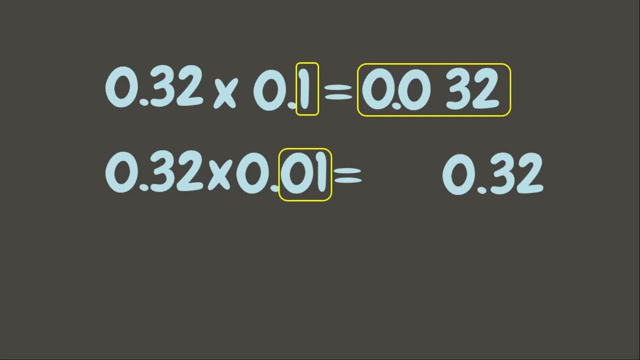 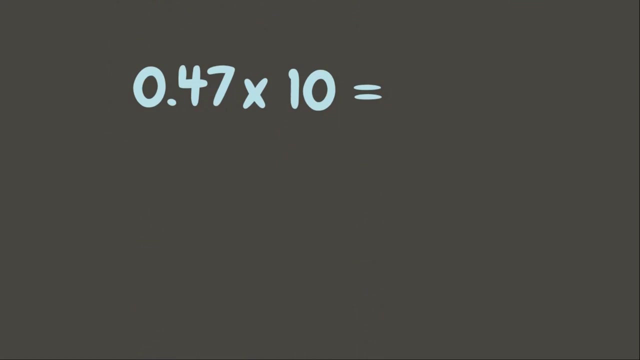 two decimal places. therefore, we need to move the decimal point two decimal places to the left. one. two: let's put 0 to the empty decimal place. there you go now. this is our answer. how about this one? let's try 47 hundredths times 10 and multiplying decimals by 10 or 100. 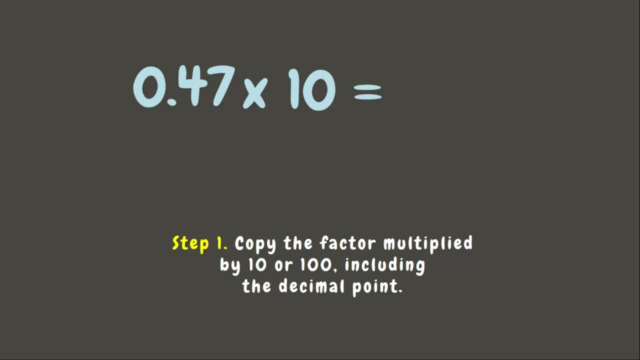 first thing that we need to do is to copy the factor multiplied by 100 or 10. let's copy 47 hundredths. now, the next step that we need to remember is the number of zeros in 10 or 100 means the number of decimal places. you move the point to the right since 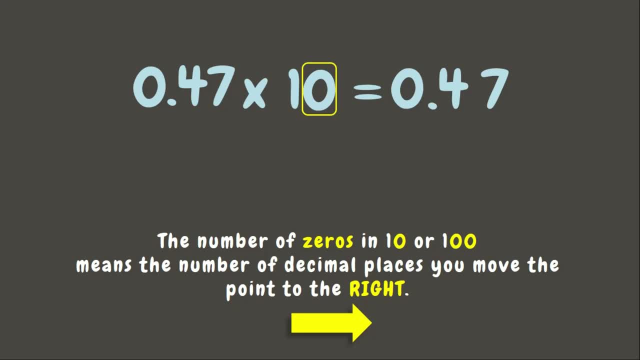 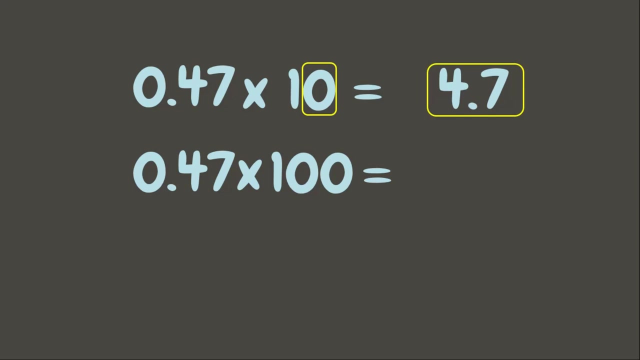 10 has one zero. we are going to move the decimal point one place to the right one there. let's just remove zero. now our answer is 4.7 or 4 and seven tenths. let's have another example. how about this one? 47 hundredths times 100. first let us copy 4,700. 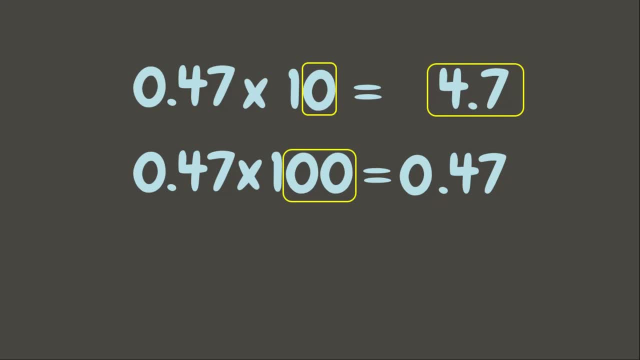 since 100 has 1 decimal place. therefore, we need to move the decimal point 2 hundredths to the left has two zeros. we are going to move the decimal point two decimal places to the right- one, two- and then let us just simply remove zero and the decimal point. 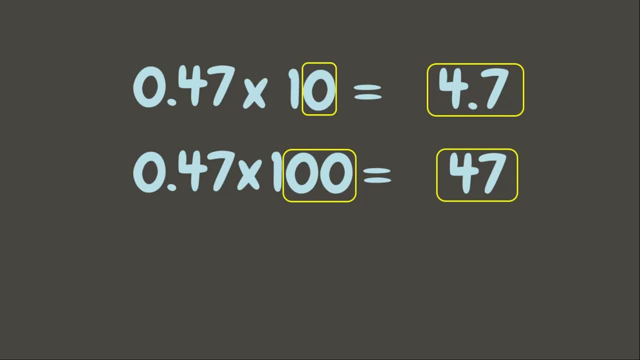 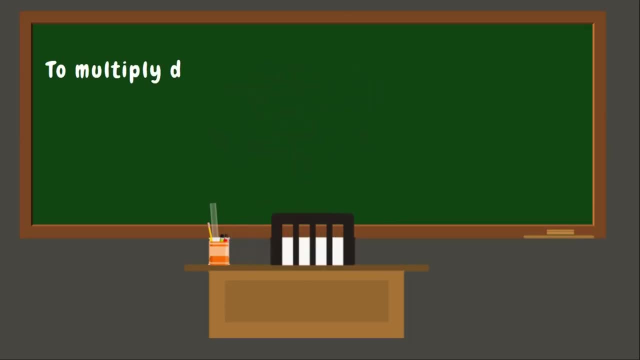 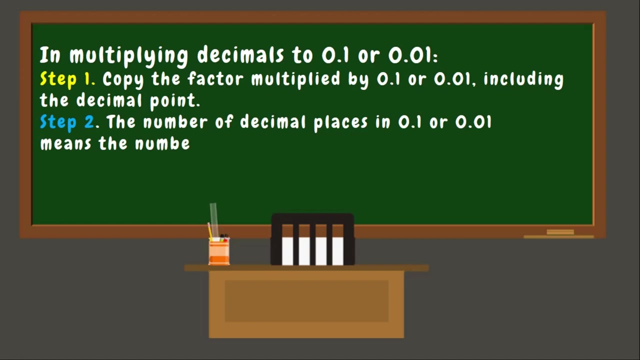 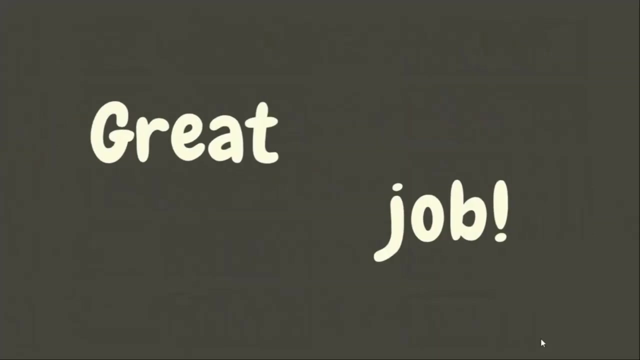 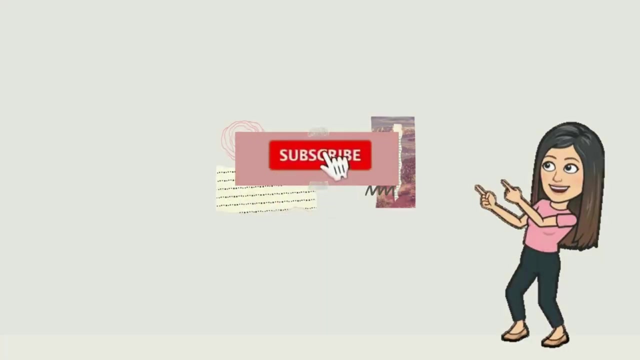 there now. our answer is 47.. great job. here are the things that you learned today, so so so.